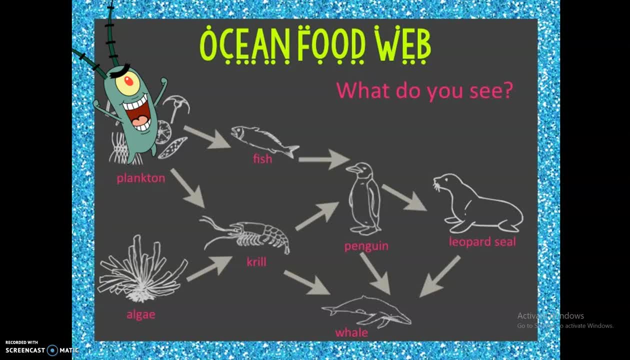 Okay, we had an ocean food web, but we have plankton here. Oh, I don't want that plankton, We need to get that out of here. Okay, sorry about that. All right, so let's start over now. Okay, so what do we see in this food web? All right, so at the start we have plankton here. Remember, the arrows point to who eats it. So the plankton saying: you know, the fish ate me and the krill They're the ones who eat me. 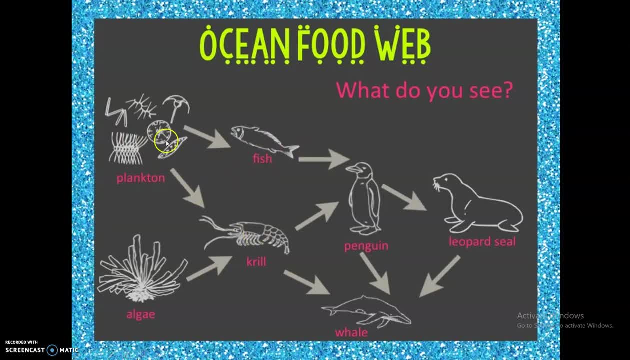 They're the ones who did it. They're my energy went to them. They took my energy. My energy goes to them. Oh, we don't have something on this food web. Where is that plankton getting its energy from? Does it just appear from nowhere? No, Where does it come from? That's right, The sun. Hopefully you said the right thing, because I'm just guessing, because I can't hear you guys. 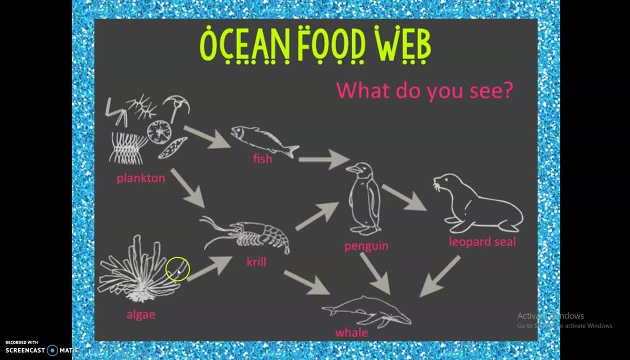 Anyway. so then we have here: the krill is also eating algae. So the krill has energy coming from plankton and energy coming from algae. Okay then the penguin: He's eating the fish and the krill. Oh, a whale is also eating the krill, So you can just follow the arrows, like so to see where their energy is going. So the top of this food web is. 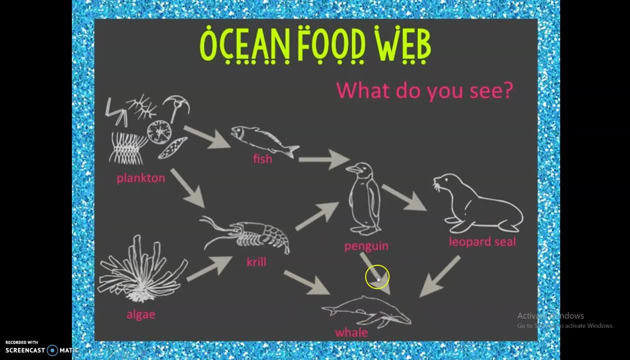 this whale because, notice at the end, everything points to him. Everything's being eaten by the whale, All right. So here's an interesting question: What would happen if plankton were eliminated from this food web? So if there are no more plankton, what do you think would happen to the fish? If the fish has, he doesn't eat anything else. What do you think is going to happen? 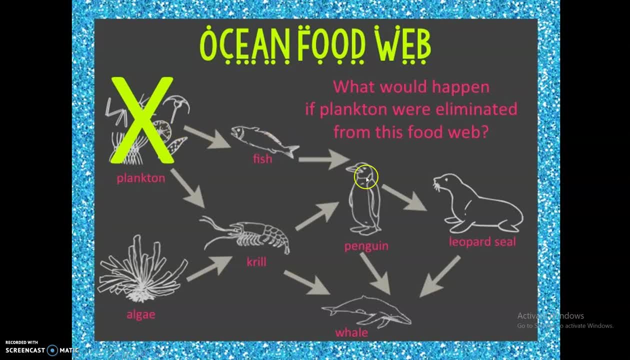 What do you think is going to happen to him If all the plankton just disappeared? What do you think is going to happen to that penguin If he can't eat fish anymore? Where's he going to have to go? Okay, so let's think about that for a second. 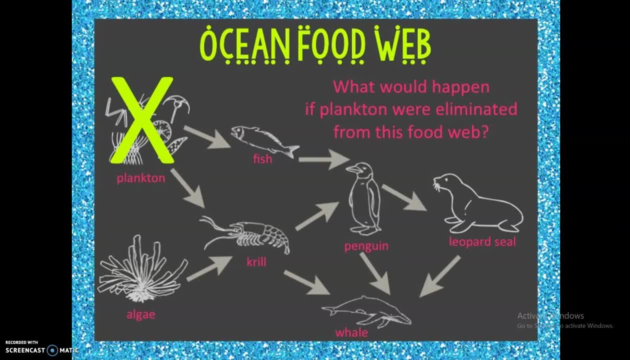 All right. So now let's see what. so fish will lose their food source. Fish would. if I don't have anything to eat, What is going to happen to me? Am I going to continue to keep living a long, prosperous life? No, I'm not. So I need that plankton. Okay, so that's going to cause the fish to suffer. If there's no more plankton- Oh, can you guys hear my dog? If there's no more plankton, there's probably going to be a lot less fish. Okay, so now let's see this krill. The krill will rely more on eating algae. So the krill's a little bit lucky. 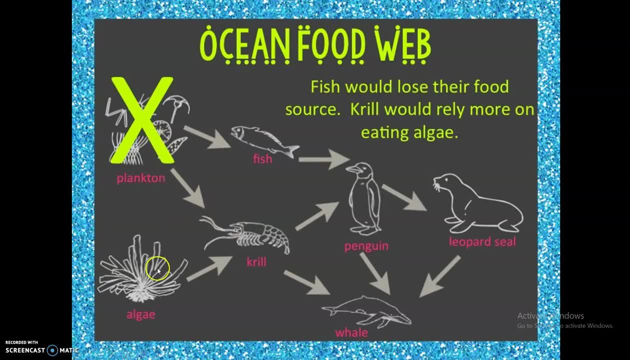 because he eats plankton and algae. so no more plankton. well, i hope you like algae, because that's all you have to eat now. so that's what the krill is gonna start eating a lot more of, all right, so again, then that's gonna fall to the penguin. the penguin is now gonna have to. 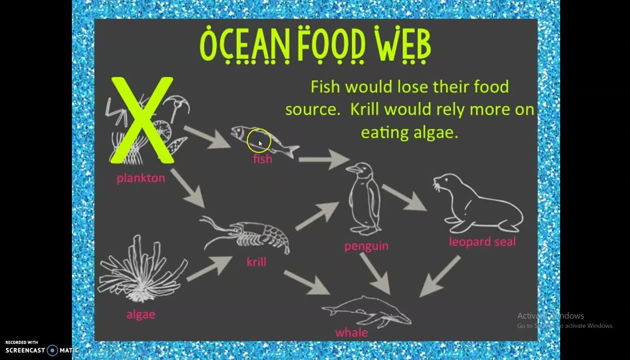 rely probably more on krill. if this fish population is decreasing because it has no more plankton to eat, okay, all right, let's try another example. what would happen if the krill were eliminated from the food web? so now there's no more krill. so i'm gonna give you a few seconds. 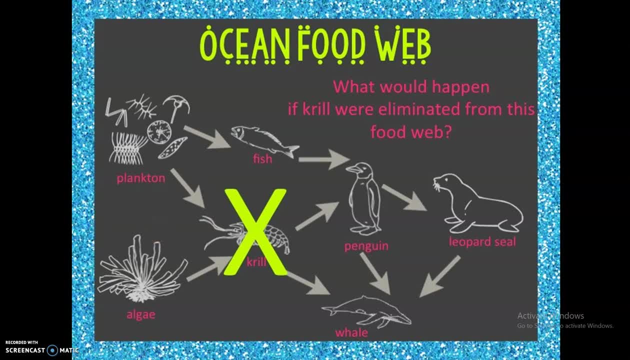 to think on that. what would happen if all the krill was eliminated? so, so a lot more algae, okay. penguins will lose their one of their sources of food. so if krill's gone, what are the penguin gonna eat now? what do they only have left to eat? that's right, the fish, okay. 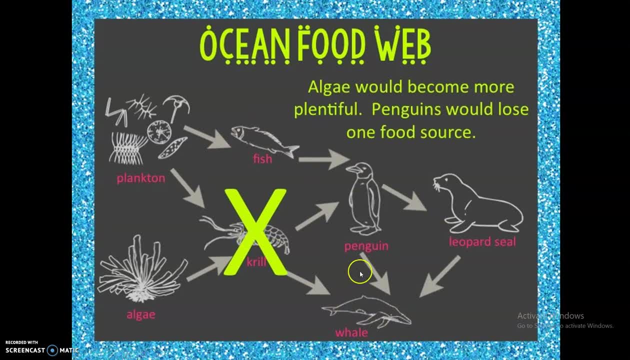 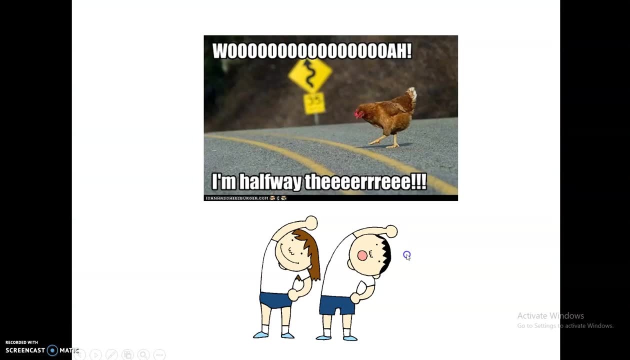 so whale also losing a food source. luckily, the whale has two more sources of food that it can eat. all right, let's move on. whoa halfway there, kind of stretch, stretch, pause. you ready to move on? okay, two more slides left. we've finished our lesson on food webs now. 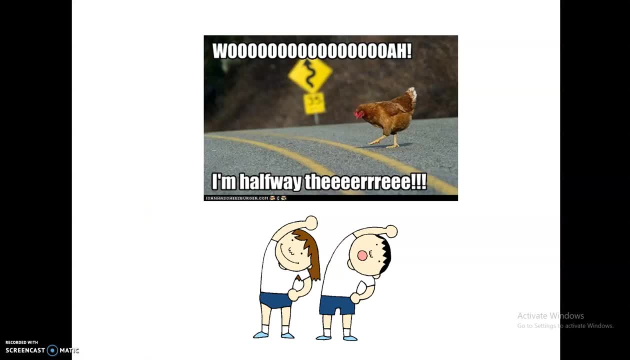 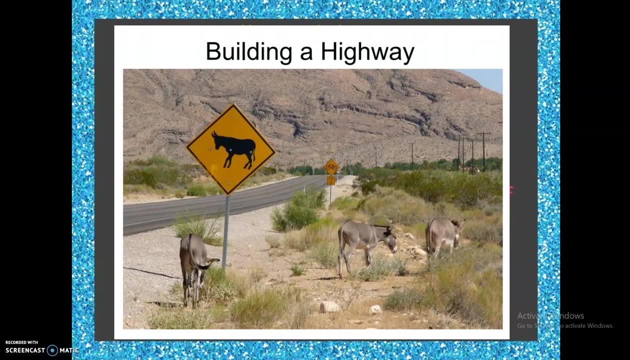 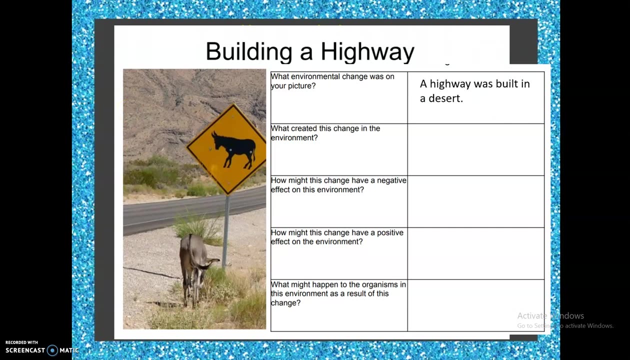 we're going to talk a little bit about environmental changes. okay, so building a highway, that is an environmental change. so what was the change? on our picture right here, we see a highway was built in a desert. what created the change in this environment? hmm, did those uh donkeys or build this highway? 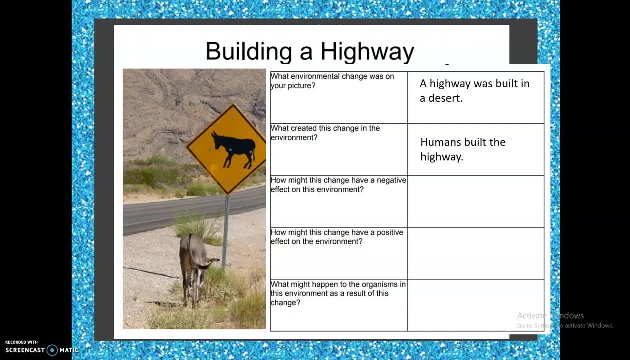 no, humans built the highway, so that's who created this change. how might this have a negative effect on the uh effect on the environment? okay, so we gotta think in the negative. we gotta be a little bit negative right now. think: how would this poor make a negative effect on the environment? 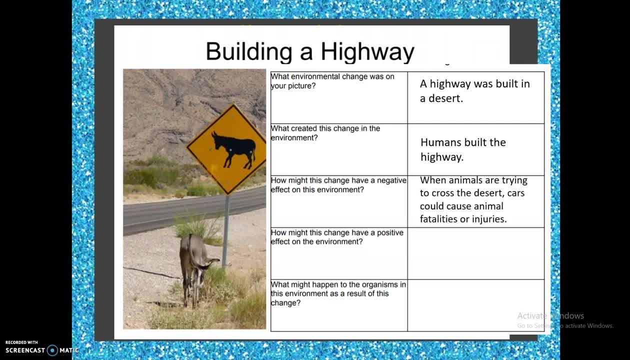 so when animals are trying across the desert, so when they're trying to walk around this place that has been their environment, they now have to compete with cars driving. okay, if their walk across at the right time and a car striving by that could cause an animal to get hurt or, even worse, have a separate fate, all right. so how might this change? 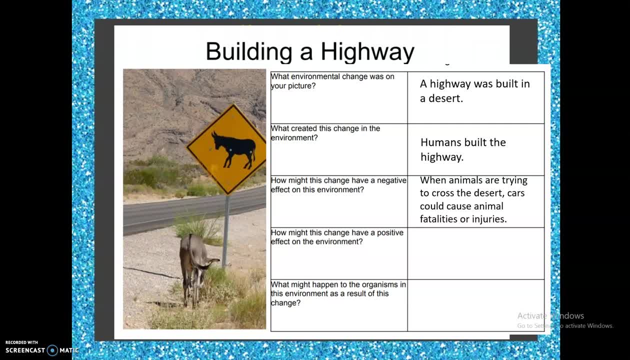 change have a positive effect on the environment. so just because we built a highway does not mean it's only negative. uh, it's only a negative effect. changes in the environment can be positive too. you have to think: okay, if there's negative, there's some way something that you can think that's a. 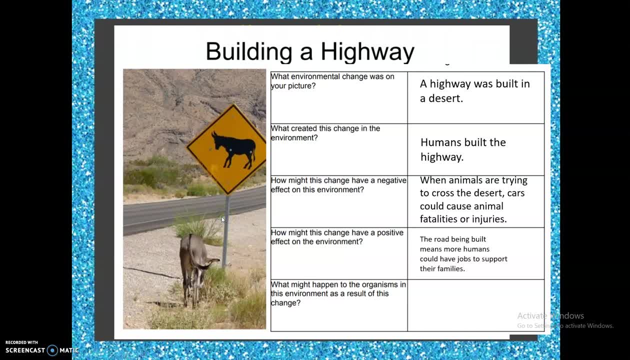 positive, okay. so a positive in this case would be that the road being built means that more humans could have jobs. we're part of this ecosystem too. humans are organisms, okay, so they could have jobs to support their families, all right. so what might happen to the organisms as a result of this? 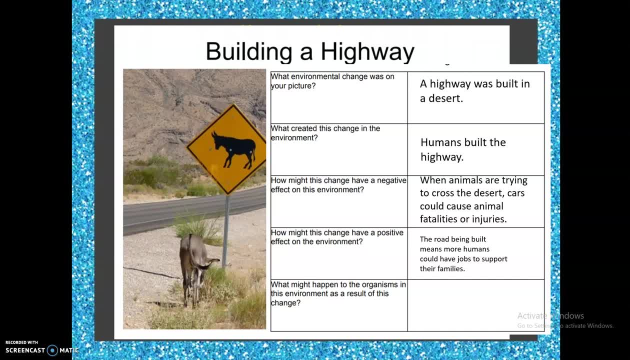 change. so think animals, humans, plants, anything like that. so those are all living things. that's what we're thinking about. human population could increase in the area. there's a road now. people can get to the stores, people can build houses along this road, okay. but if that happens, that also means 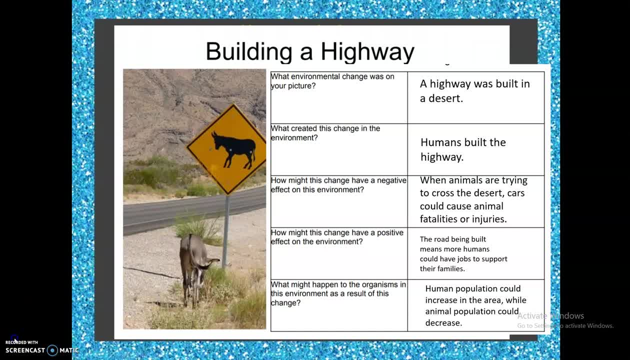 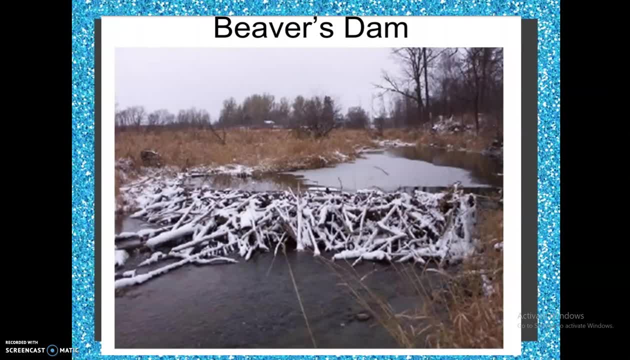 that you, you animal population, could decrease. all right, guys, could you hear my dog crying? she was upset that i was talking and not paying attention to her, but i think she's gonna take a nap now, so we should be good. so let's move on to a beaver's dam. okay, so this is right here, a beaver's dam. so this is where. 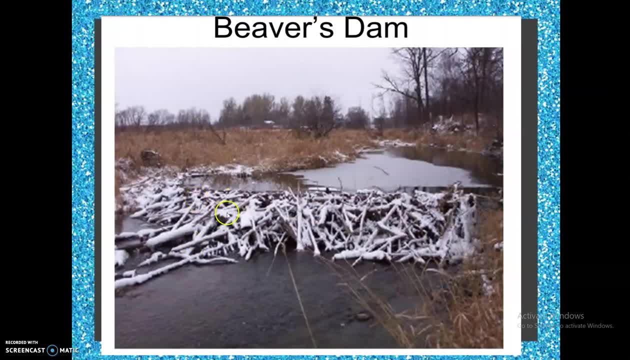 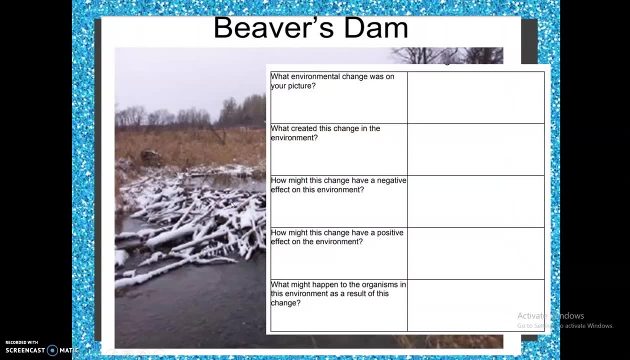 they pile up a whole bunch of logs and sticks and parts of the tree, and they do this in a river. okay, so what environmental change was? on this picture we see the beavers built a dam and it actually blocks the river from flowing. okay, so it's not that strong current that usually goes. 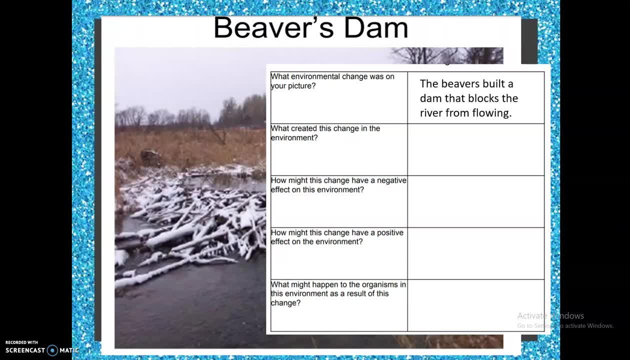 through? what created this change in the environment? okay, so, believe it or not, humans did not go in there and make that pile of sticks. the river flowing didn't. just that wasn't erosion that made that, that pile of um tree branches. so the beavers actually built this dam. okay, how might this change have a negative effect on the? 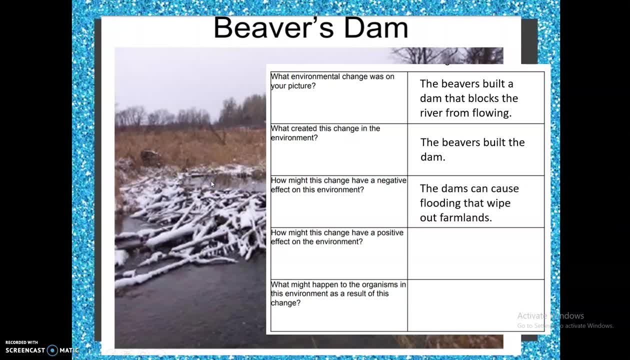 environment. okay, these dams can cause flooding that wipe out farmlands. okay, so that's kind of a negative effect that it could have on us as humans. okay, so if crops are being destroyed, things like that that would hurt, um, the humans in this environment. okay, so some things have negatives, some things have positive. 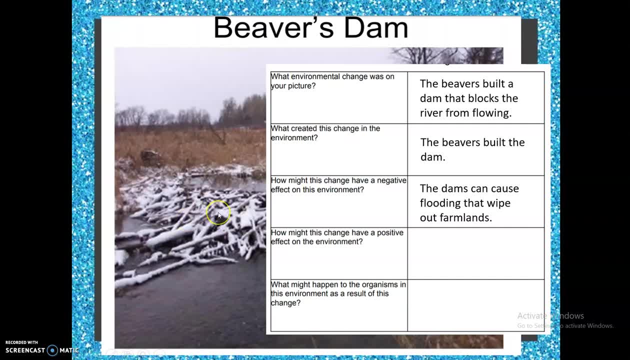 right. changes can be both all right. it's not just, oh, it's always negative. no, sometimes it can be both. so how might this change be a positive effect on the environment? so i don't know how much you guys know about beaver dams, but i want you to kind of think: how could this have a positive effect? 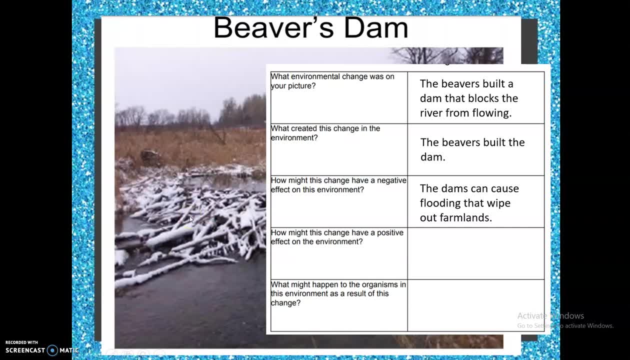 on the environment. all right, so the dam acts as a natural filter so it can actually stop some bad stuff from flowing, continuing to flow through the river and getting into our ocean. so that can actually help some of the other animals, not only in this environment but in that ocean environment also. okay, so that's. 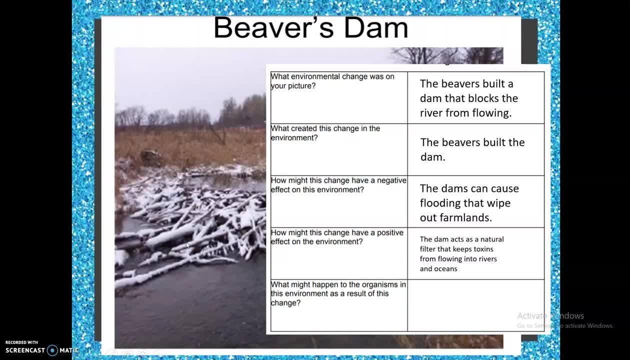 something pretty cool about a dam that i didn't know until preparing for this lesson. so the last one is: what might happen to the organisms in this environment as a result of this change? so i want you to think. you pause the video for a second, think. how could a beaver's dam help or hurt, maybe even. 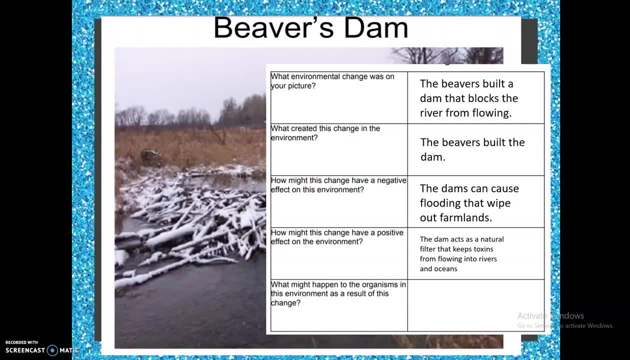 the other organisms in the environment. okay, all right. well, this is the end of this video. i hope you enjoyed it and i'll see you in the next one. thank you so much for watching and i hope you enjoyed this video and i'll see you in the next one. 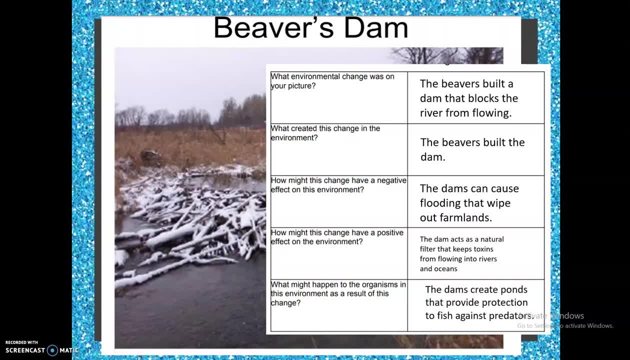 so the dams create ponds that provide protection to fish against predators. so this may be something that you didn't know, but since it's blocking the river, it creates a pool of water on the other side, kind of like a pond, and that makes it harder for predators to hunt fish. okay, so these dams? 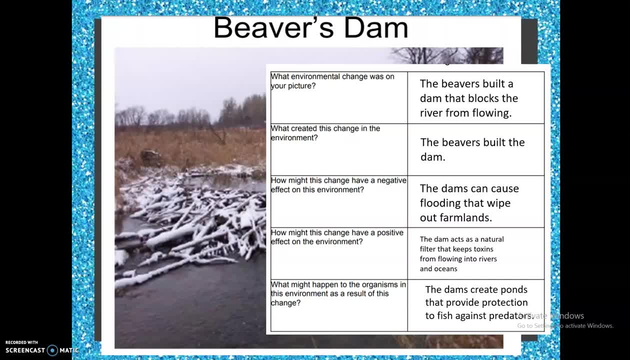 actually, if no, if it's harder to hunt the fish. it's harder to hunt the fish. so i'm going to show you the fish. what do you think is going to happen to the fish population? that's right, it's going to increase. okay, so it'll keep going up. the fish will continue to live and reproduce because the 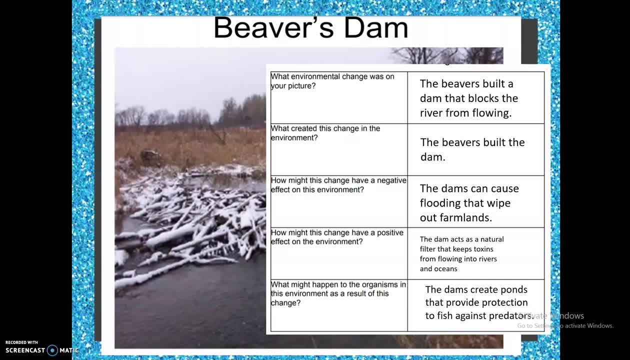 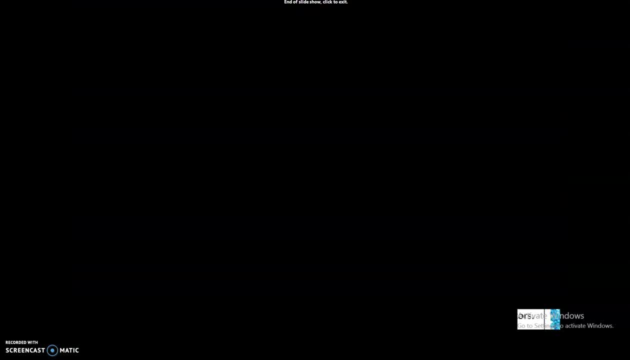 predators are, it's harder for them to get to it. okay, all right, you guys? well, that is everything i have for you. i want you to do the discussion below, so pick one of those sentence stems below this video and type in, fill it in and have that as your response. that's my. 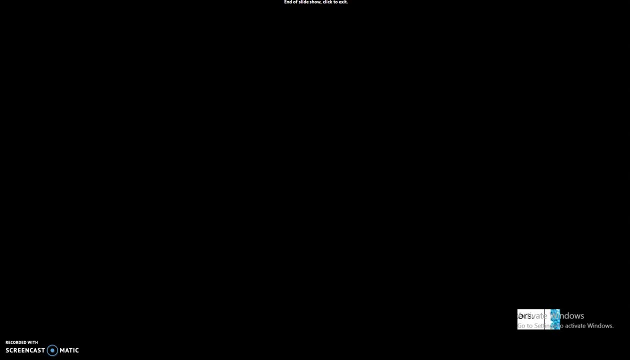 check to know that you watch this, and that's kind of like your exit ticket to do the next thing. okay, you need to complete all your must do's by the end of the week. i'll give you until sunday to have everything done, okay, so if you want to try and power through, get it all done as soon as possible.